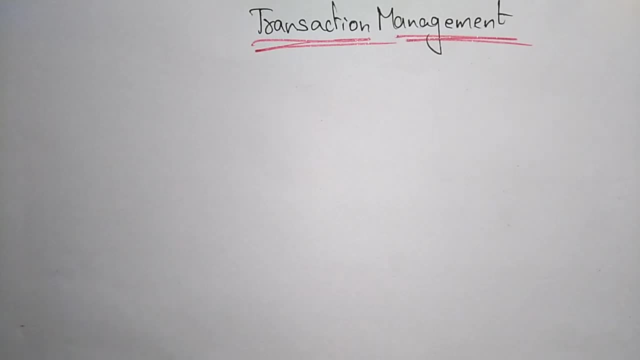 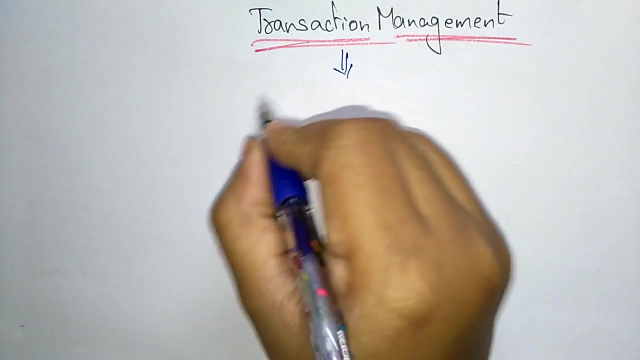 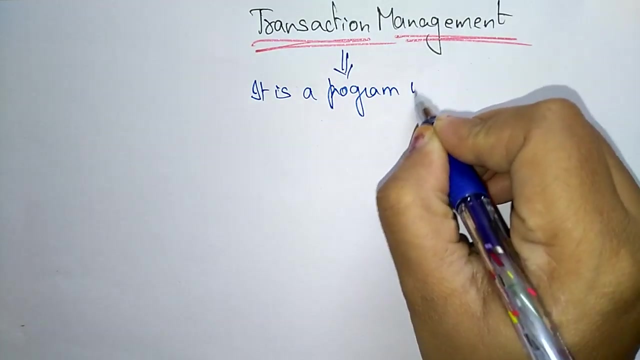 Hi students, welcome back. Coming to our next topic, that is, transaction management. So let us see what is this transaction management in database management system? So if transaction management is nothing but it is a program unit You call, it is a program unit whose execution 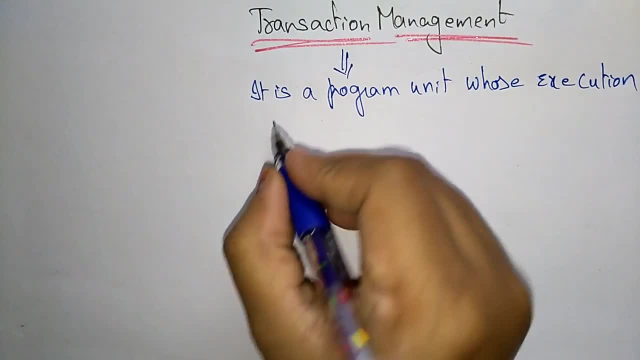 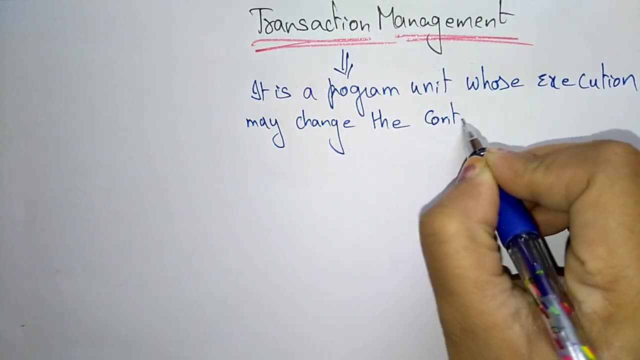 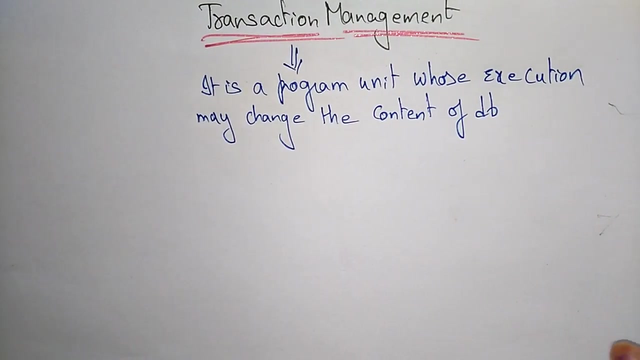 whose execution may change the content of database, So that you call it as a transaction management. So here the transaction management is a program unit whose execution may change the content of database. So what it means? what is the whose whose execution may change the content? 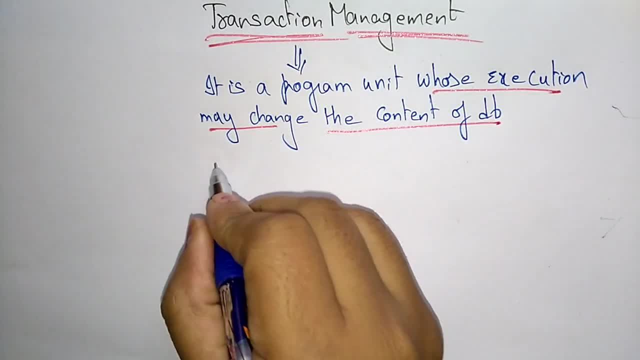 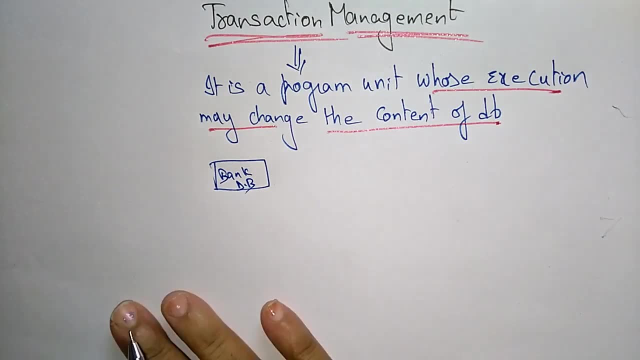 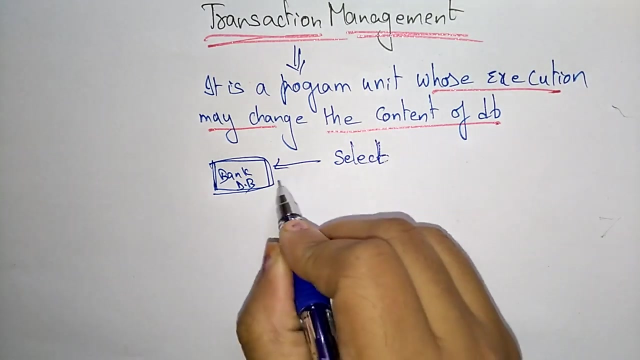 of database. suppose you are having one bank, database is there. so in a one particular bank you are having some account, so database is there. so here the transaction means whose execution may change the content of database. so how this database content will be changed with the help of some select. you are selecting the database and you are doing some insert by using insert. 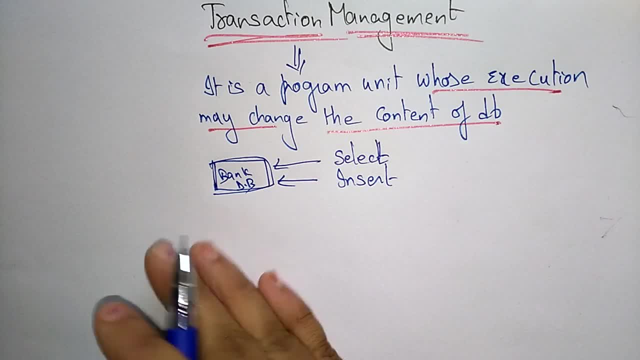 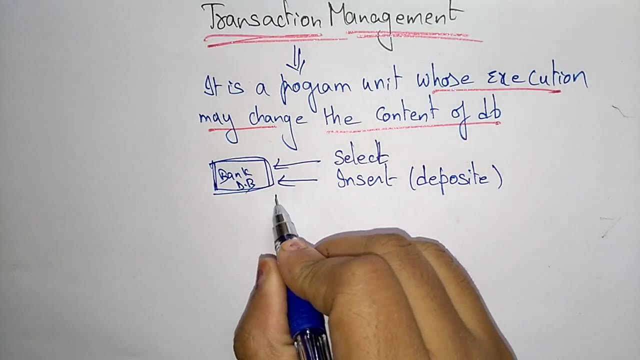 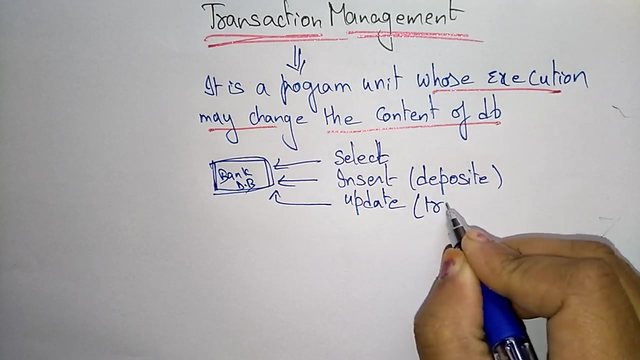 operations means you are transferring the money to the bank. okay, you are depositing the money deposit. so whenever you deposit the money in the database in your account, the content of database is changing. so that is one of one type of transaction. suppose if you update, you are transferring the data from one account to the another account. okay, so here also. 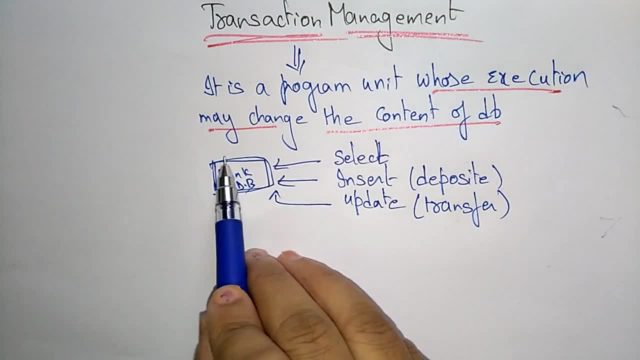 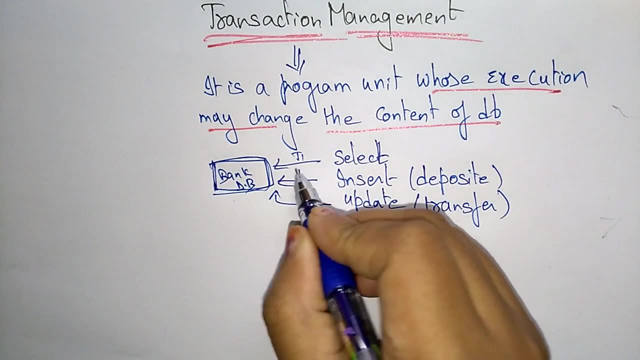 whose execution may change the content of database. the database content is changing so that you call it as a transaction. so selecting one type of transaction- inserting the account amount, depositing the amount in your account- is changing, changing the content of database. so that is one type of a transaction. 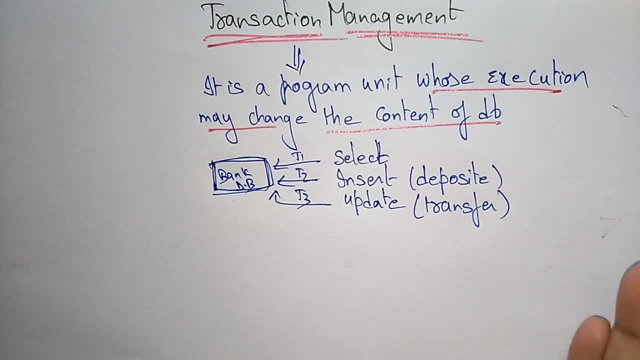 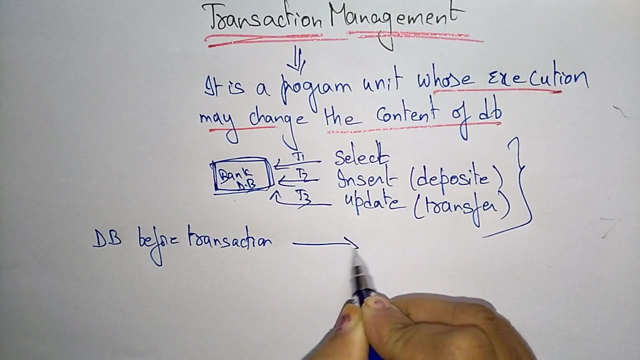 and updating the account by transferring that amount from one account to another account. so these are all the operations that are used to change the content of database, so those you call it as a transactions. so doing a simple operation you call it as a transaction. so a database before a transaction and the database. 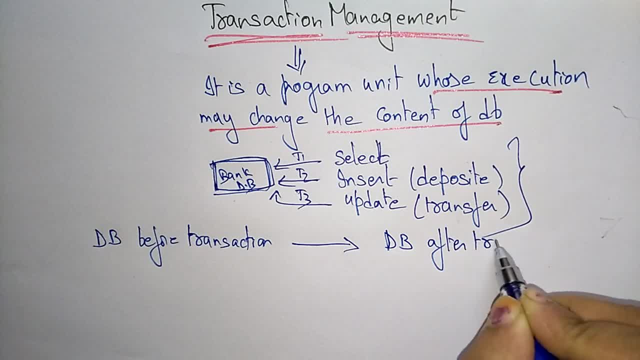 after transaction: okay, after transaction. it should be. same means it should be consistent. then only you can say the whatever the transactions you made on the database is valid. okay, database before transaction and after transactions. it should be in consistent state. it should be in consistency. actually, the consistent state is: 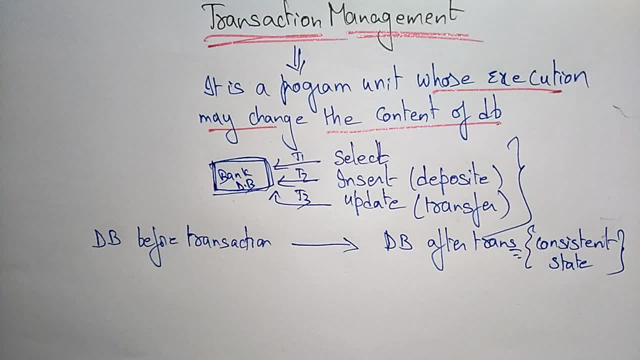 nothing, but it is a correct, consistent means the correct values or the correct database. okay, so database before transaction. so before transaction and after transaction. also it should be in consistency how it is, in consistent state. so let us see the example. let us do one transaction. okay, suppose in your account you are having the money in your account the amount will be: suppose 300 is. 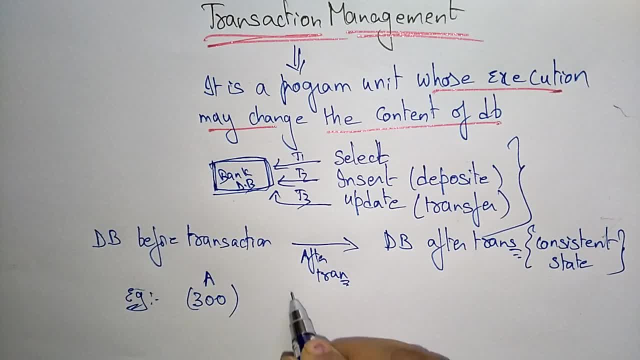 the amount in your account, account a. so in another account you are having the amount in your account. so in another account you are having the amount like: okay, so 400. so in another account the amount you are having the four, uh, 400. now you want to transfer the 100 rupees, 100 rupees from. 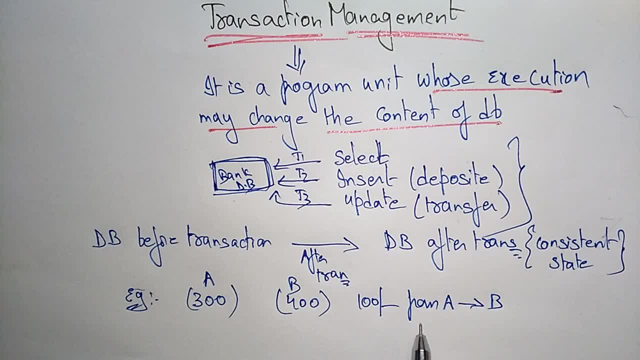 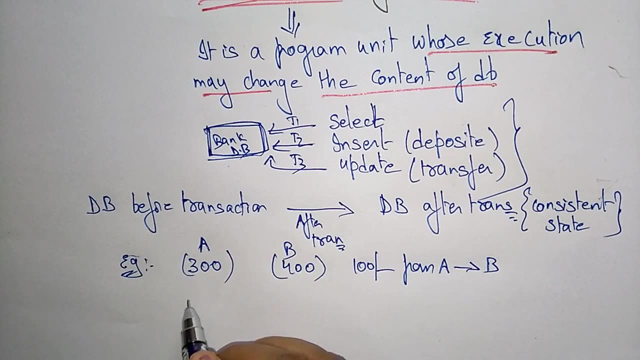 a to b, so from a to b, from account a to account b, you want to transfer the money, 100 rupees. you want to transfer means you want to do some transaction on the uh database of your account. okay, so transferring, modifying the data, so how? first, read a r means, suppose, read a, so 300 is. 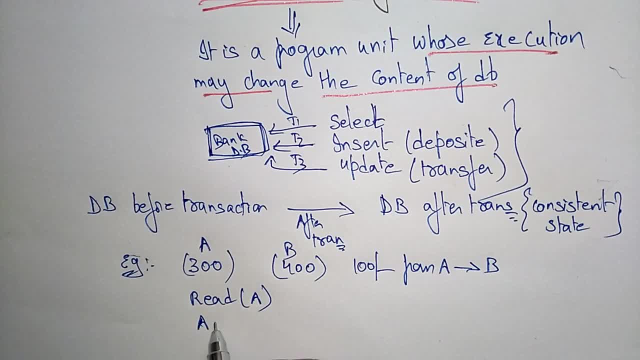 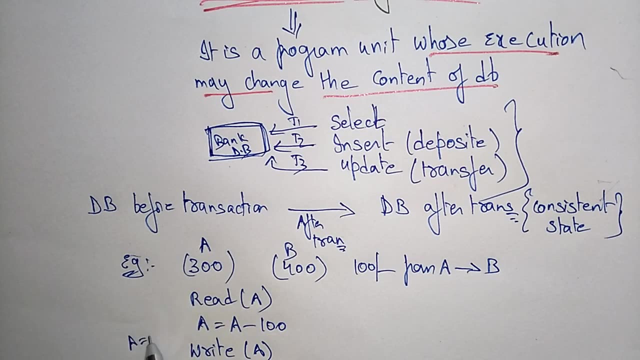 read. so after that you have to be a minus 100 means you are transferring the 100 amount, so 100 will be deducted from your account and write a. so now your account is having 200 transfer the amount. so after that read b. okay, 400 is read, b is equal to b plus 100, because the 100 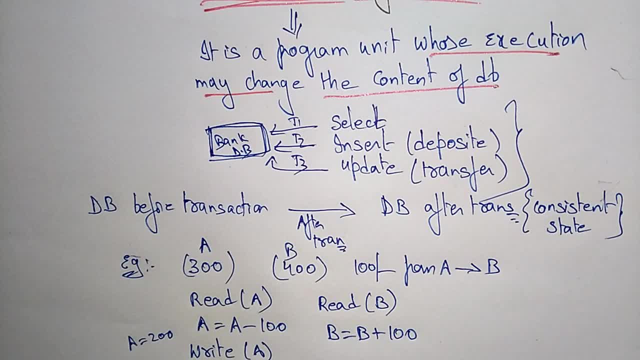 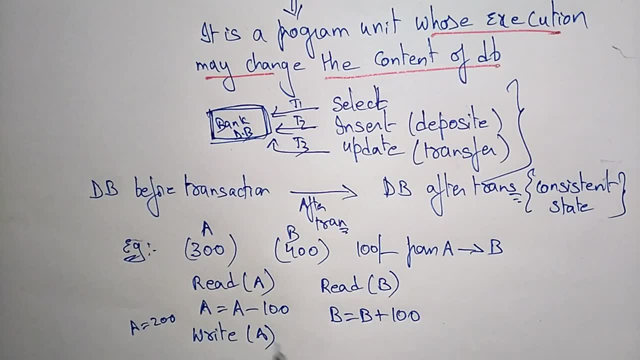 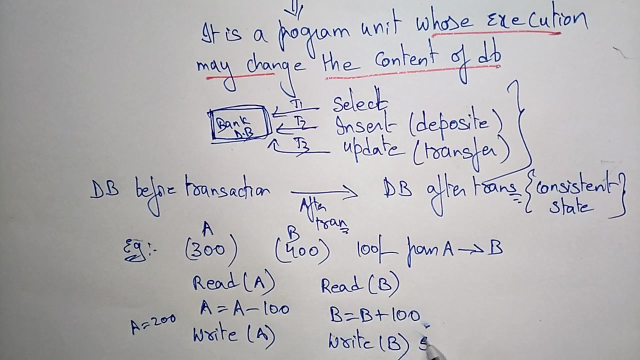 is taken from account a, the amount is transferred. so this is a general uh mathematic problem. so here we are just adding the uh removing the hundred rupees, we are transferring hundred rupees to b. so now b is equal to b plus 100.. now write b. so now b value is 400 plus 1 500. okay, so here you have to observe before transaction the: 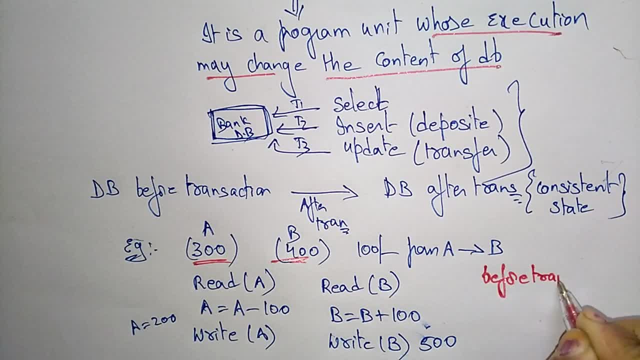 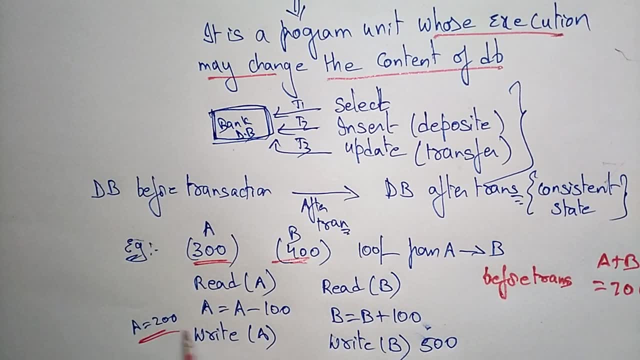 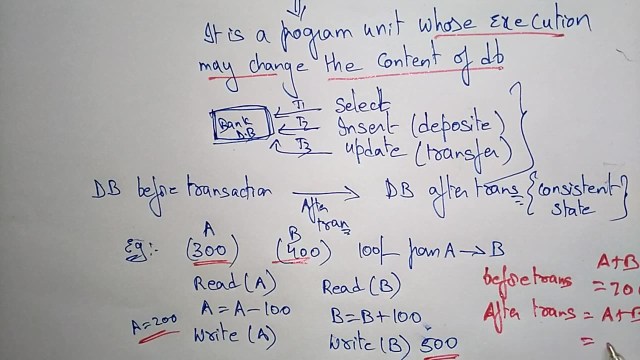 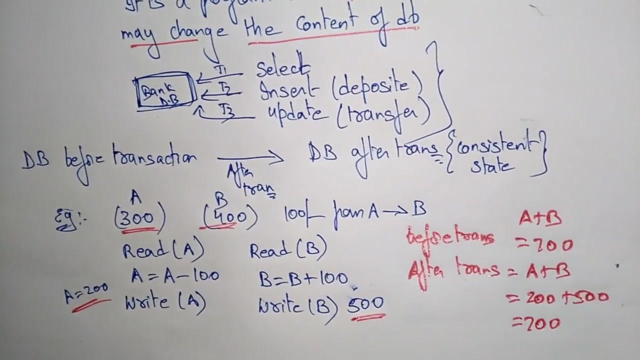 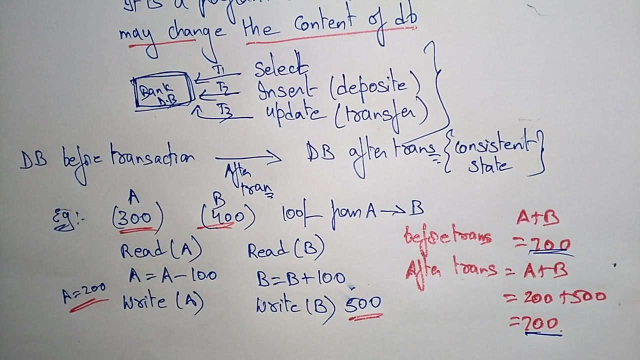 account value before transaction a plus b is 700, 400 plus 300.. so after transaction, after transaction, a plus b, that is 200 plus 500, 700. okay, after transaction a plus b is also 700. then you can say the database is in consistent state without any uh problem. okay, so before transaction, after. 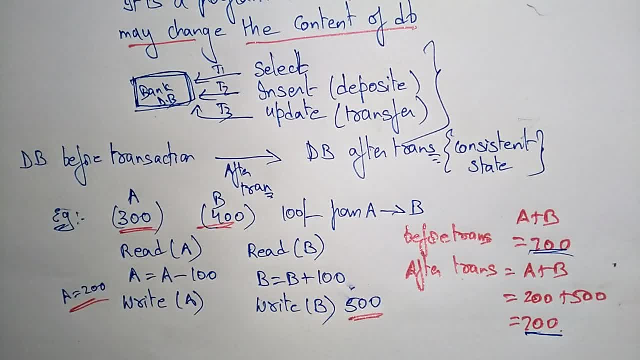 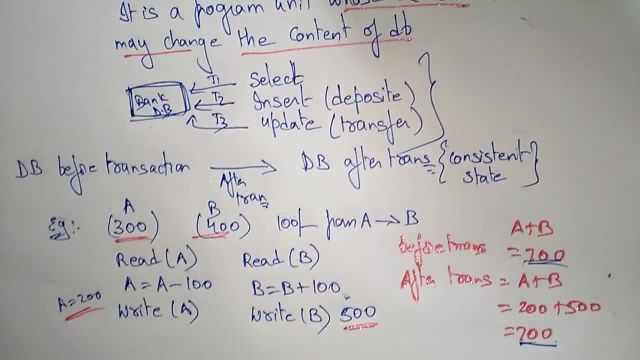 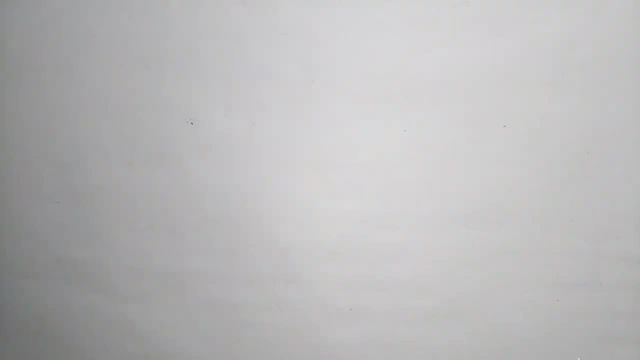 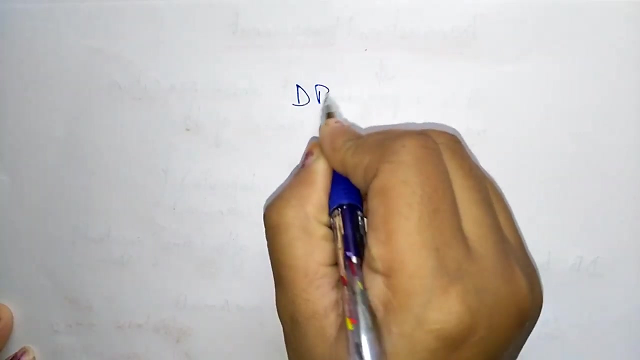 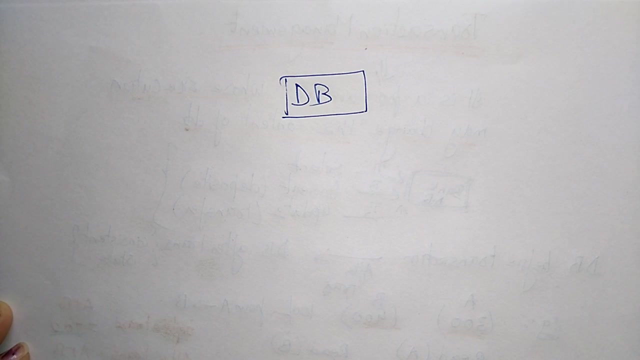 transaction. the database should be in consistent state. to make the database into consistent state, we will use some properties on transaction. so actually, whatever you are created- okay, suppose, whatever you are created, uh, a database- that always in consistent state. okay, first you created a database, so that database is always in consistent state, it is in correct state, okay. so now what we have. 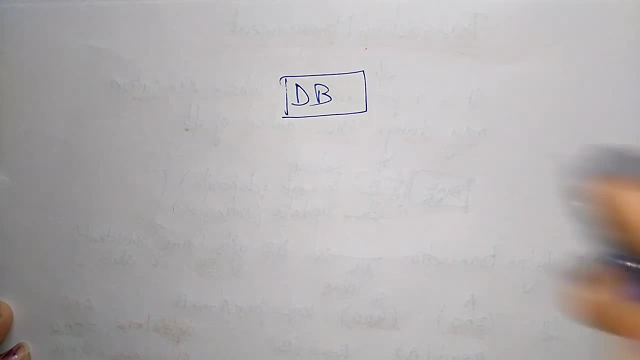 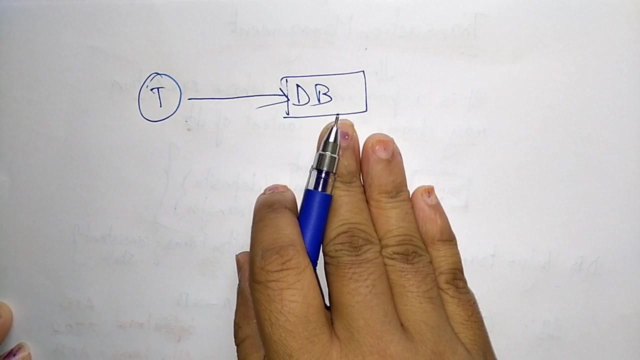 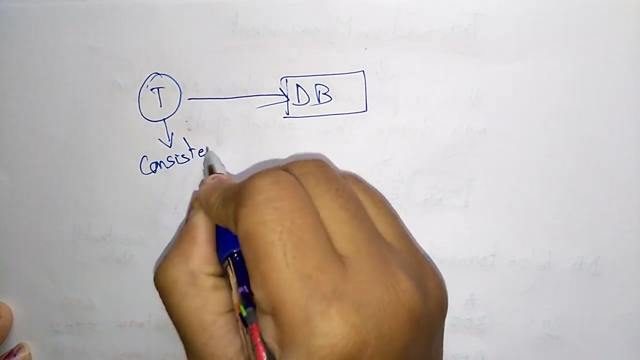 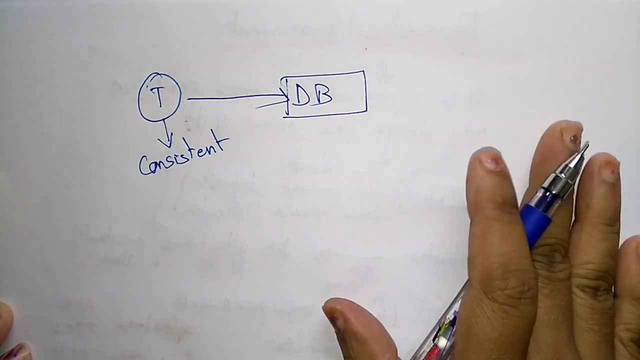 to do the main thing here, we have to note that the transactions that are doing on the database, the transactions that are we are, uh, doing on the database, should be consistent. so, whatever the transactions that we are making on the database, like select, update, delete, modify, okay, commit- so all the transactions that are we are doing on the database should be always. 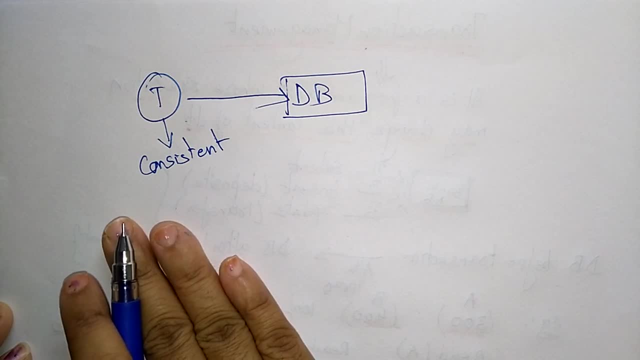 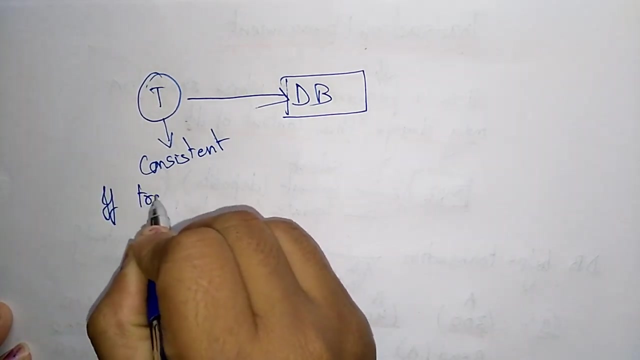 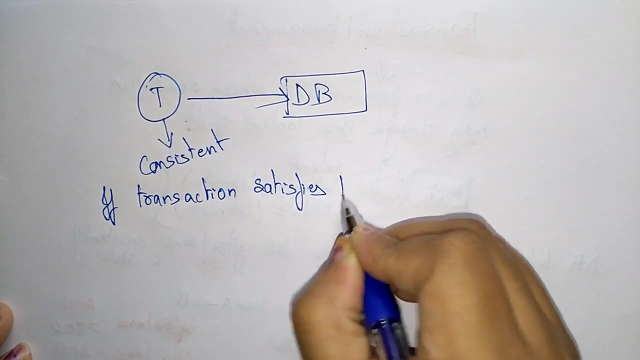 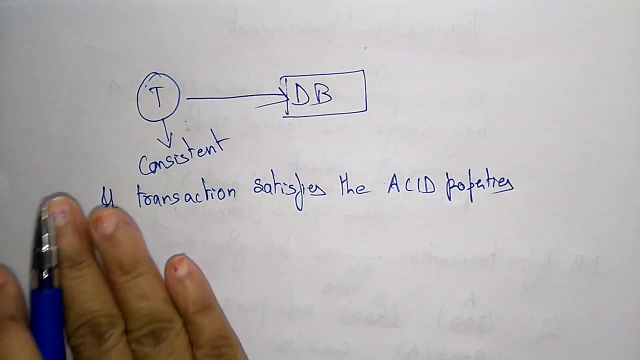 in consistent. that we have to be noted. okay, so to make the transaction into consistent, consistent state, we will use some properties- okay, those you call it as acid properties- if transaction satisfies. if transaction satisfies the acid properties, then you can say that your transaction is maintaining database consistency. okay, so if your transaction satisfies all the acid properties, 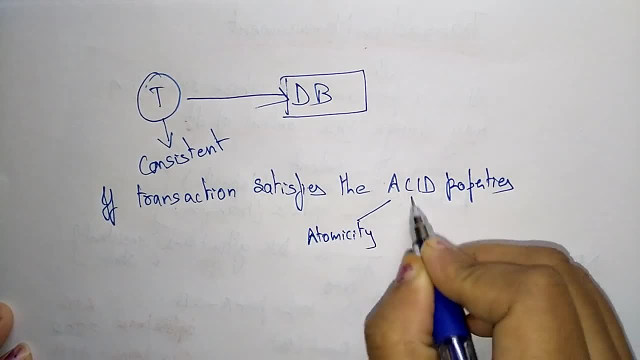 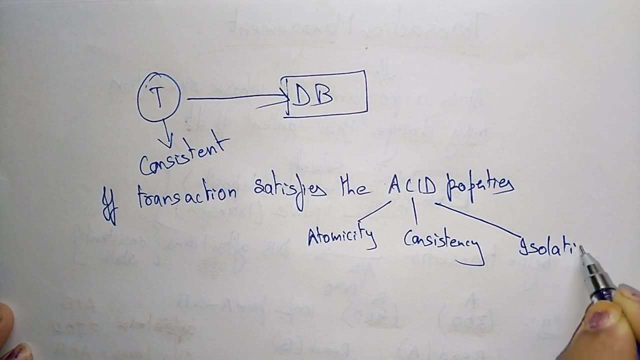 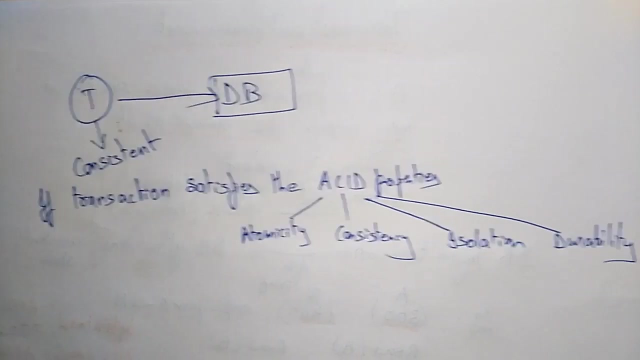 atomicity, consistency, isolation and durability. so these are all the different acid properties. so if your transaction satisfies all these acid properties, then you can say that Transaction Satisfy. Haha, оказ під spheres bater Corpsowatra numaMoña conserv PDS. 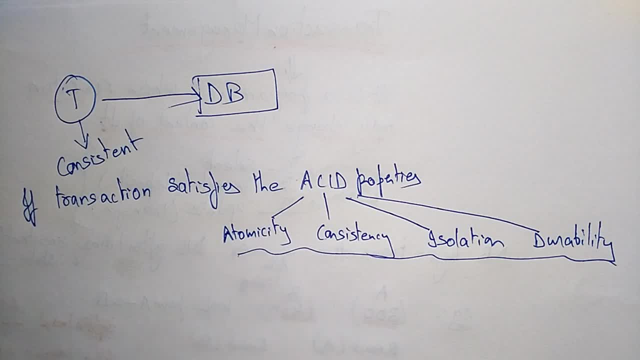 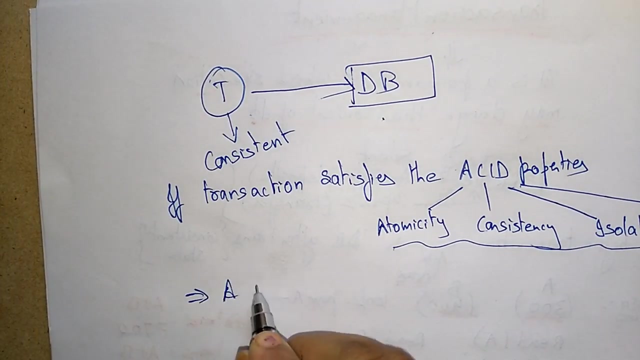 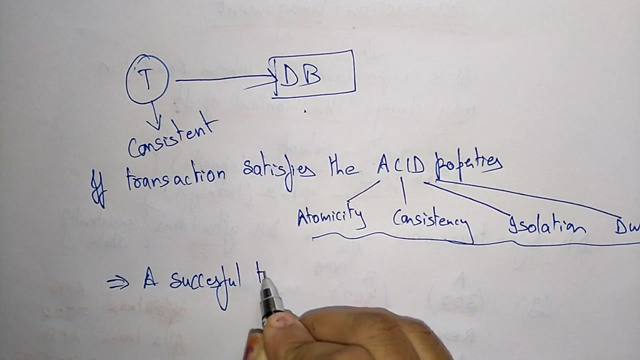 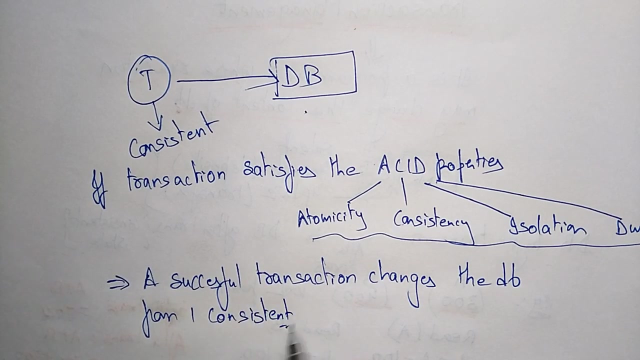 transaction, whatever you are doing on the database, is consistent and it makes your database in a consistent state. so the successful transactions always change the database from one consistent state to another consistent state. okay, a successful transaction changes the database from one consistent state to another consistent state. so this is the transaction, so this is the transaction management. 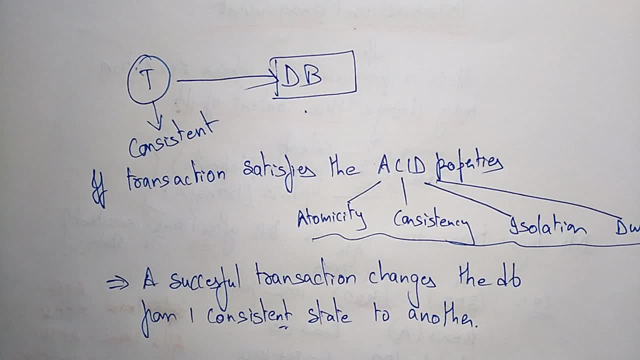 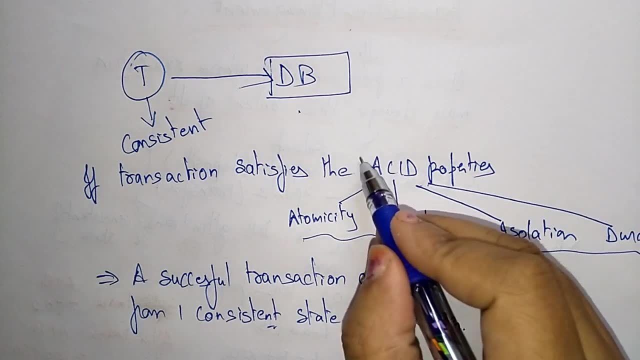 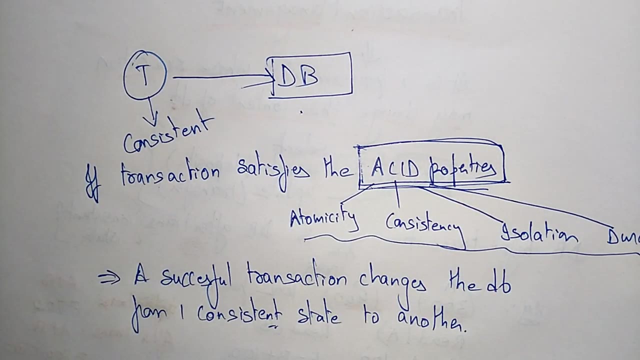 to maintain the consistent state of the transaction. so this is the transaction management in the transactions, whatever the transactions that are, we are doing on the database. to maintain those transaction as a consistent, we have to satisfy the ACID properties. so we will use the ACID properties. so, with the help of the ACID properties, we can ensure that, whatever the 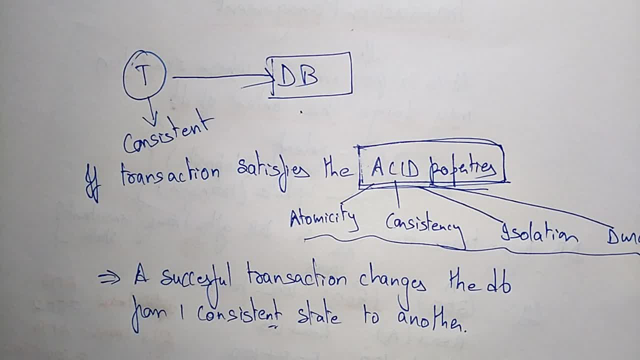 request we are giving to the database. that should be in consistent state. thank you,